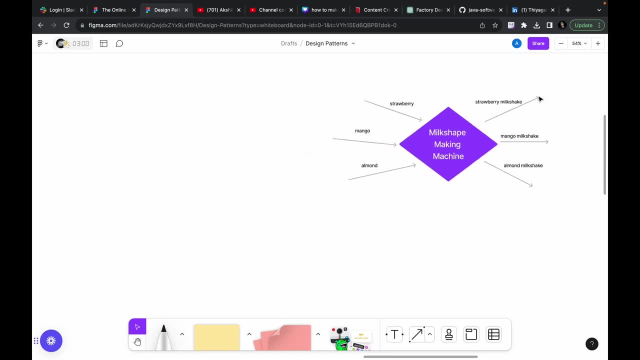 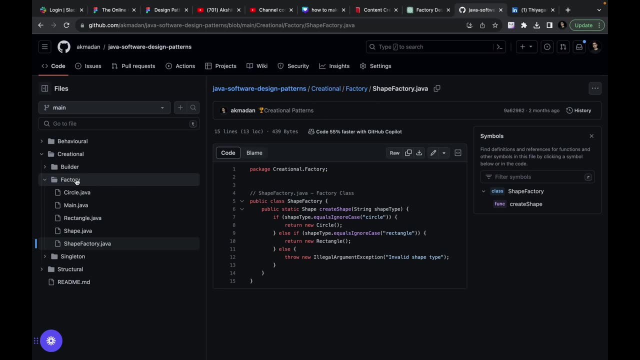 and you get an output object. You get an output right Now. let's take a code example. I have created a factory package inside my creational package. Now, inside this factory package, I'm having some classes And we are going to explore these classes one by one. 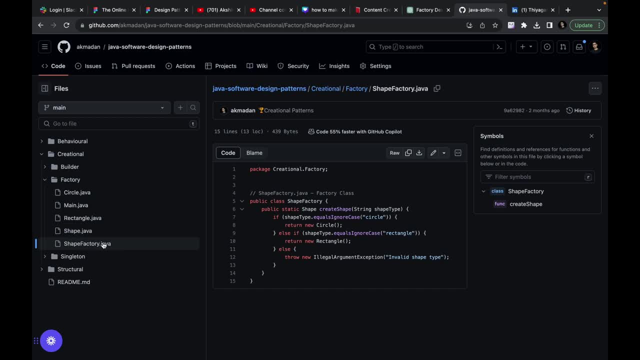 First of all, let's explore our factory class. So we have shapefactoryjava, So basically we are creating shapes. in this example, We are going to create circle, We are going to create rectangle using factory design pattern, not a normal class and object, and 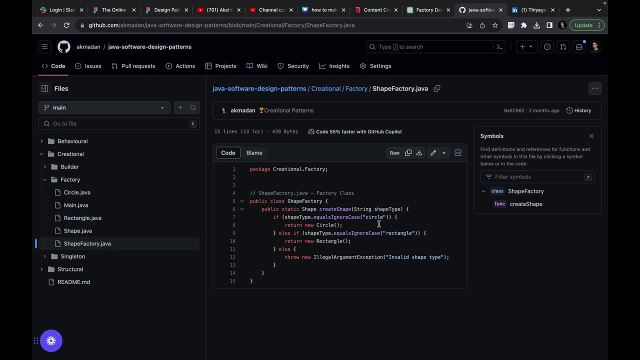 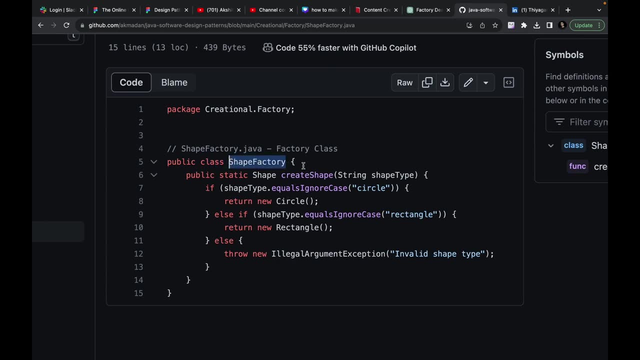 instance method, right? So first of all, I have a shapefactoryjava right Now. inside this shapefactoryjava, consider it as a factory class, right? If it is a factory class, that means it is going to help us create some objects based on the input that we have provided, So it has a 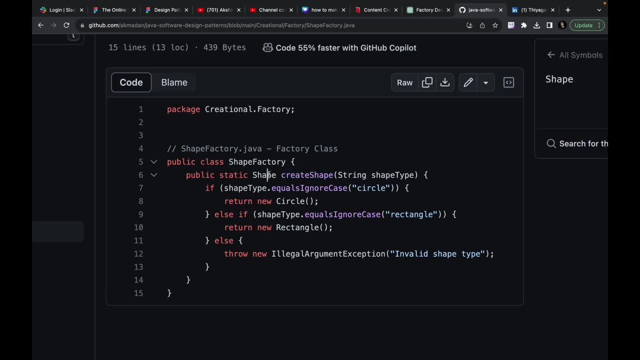 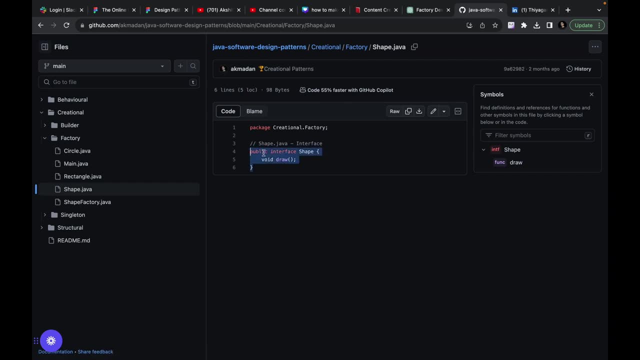 static function: create shape. This is a return type of shape. Now, what is shape? Shape is another class that I am having over here. The shape class only has. it is a public interface and it has only one implementation of a draw method or a function. right, Not an implementation, but definition of my. 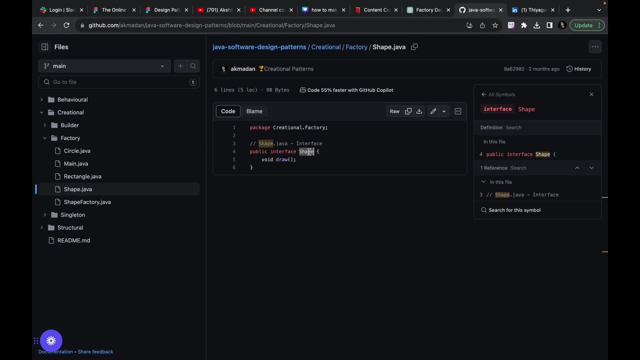 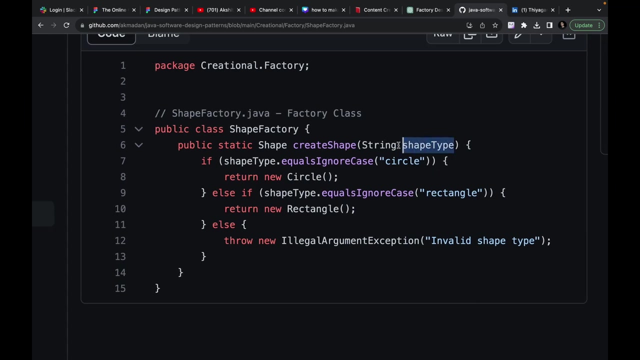 draw function. This means that every shape, every child of my shape class, that means every class that is going to implement this shape class, is going to have a draw method. That's it Coming back to our factory class. Now, inside this function, what is happening? It is going to take a shape type in the string as a string format and it is going to check if it. if the circle is provided as a shape type, I'm going to give a circle object. If rectangle is provided, I'm going to give it a rectangle object. That means I'm creating objects based on the input that I'm getting. Consider it as a strawberry: I'm providing strawberry. I'm getting strawberry milkshake. 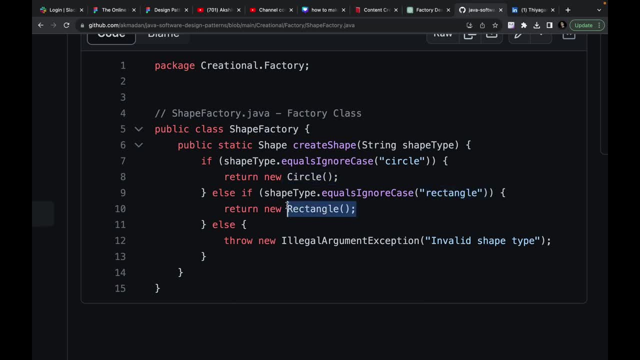 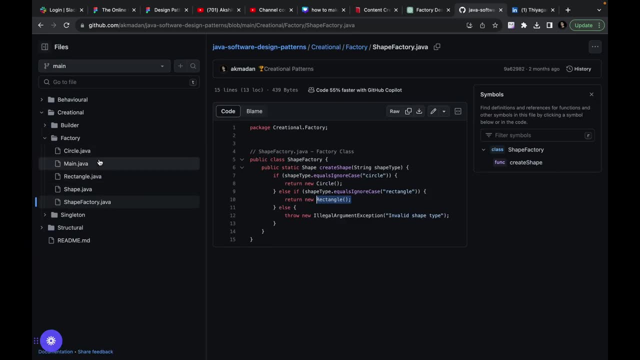 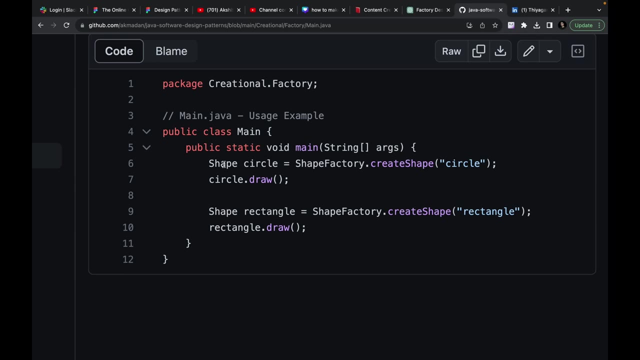 I'm providing mango, I'm getting mango milkshake, right. Other than this, it is invalid shape type. That's it Now coming back to our mainjava. In the mainjava, what I'm doing in the main, function: shape circle. shape circle, that means class name, my object name, shape, factorycreate shape, And I'm providing the parameter circle. That means my factory class is going to create a shape as a circle shape.